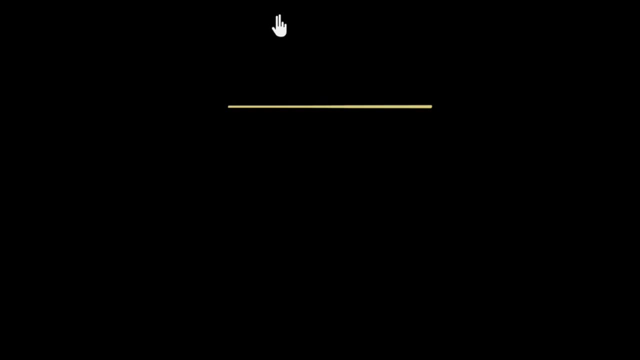 we need to understand a very important thing. The most crucial thing to understand is the idea of work function. So let's take an example. Imagine this is gold And I looked up online. it turns out the work function, which is often represented by the symbol phi. 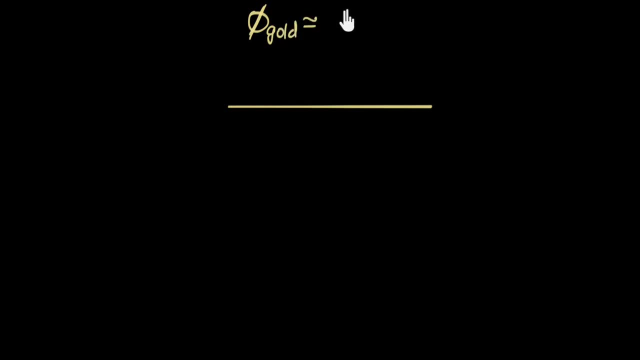 the work function of gold happens to be somewhere around five electron volt, though. So the question is: what is the meaning of this statement? Well, first of all, what is this electron volt? It's a unit of energy. Let me write that This is a unit. In fact, it's a. 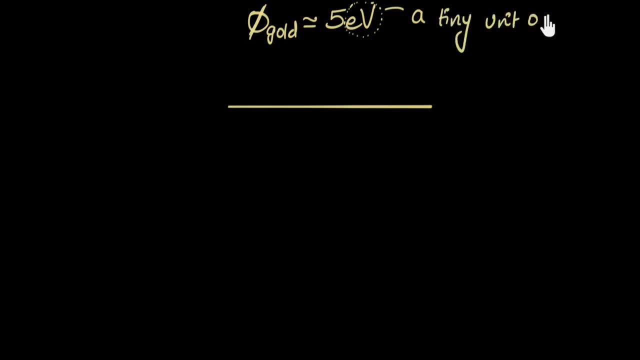 tiny unit of energy. just like how, when we're dealing with very tiny masses, like mass of an atom we are using, we don't use kilograms right, because it's very small, so we use a different unit like atomic mass unit, right. similarly, when we're dealing with energies of electrons or 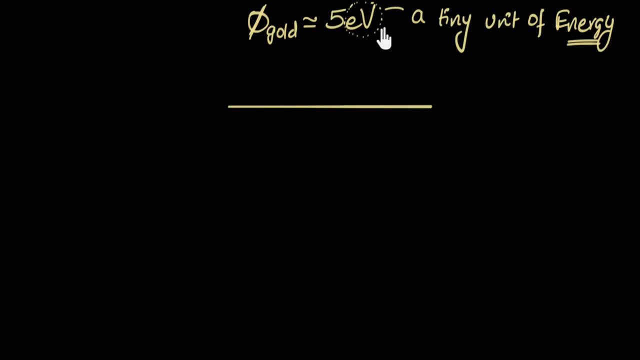 photons, because those energies are very tiny. we don't use joules. we came up with a new unit, a very small unit, which we call electron volt, and of course we'll talk more about exactly what it is, its connection with joules. all of that we'll do in the future videos. but again coming back to the 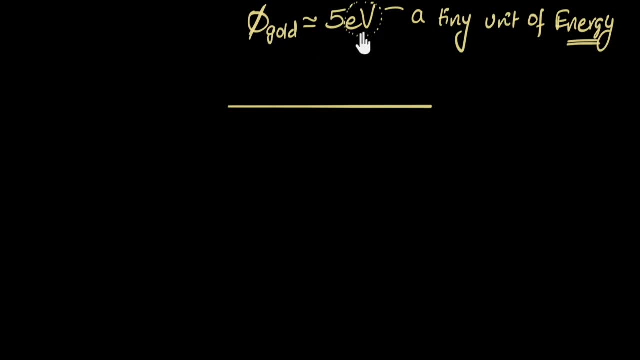 question: what does it mean to say that work function of gold is five electron volts? well, the gold, gold metal has electrons inside of it right now. if you want to pull that electron out, then it doesn't happen for free. you have to spend some energy because this electron is attracted by. 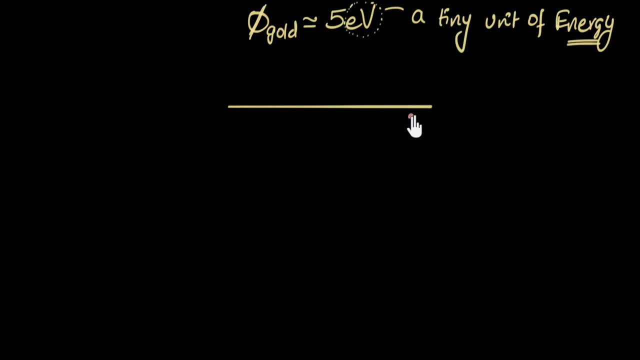 the different you the positive nuclei right, and so you have to spend some energy. so this number tells you the minimum energy needed to pull an electron out of gold. so let me write that this represents minimum energy, minimum energy needed to pull an electron from gold. all right, so let me draw a few. 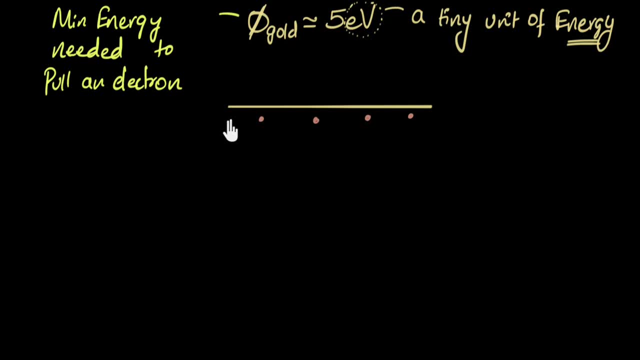 electrons over here and now our stage is set. and now let's say we shine some light on this. so let's say we shine I don't some light, I'm gonna use some color. don't take that color very seriously. it's not the exact color of light. but let's say I like I shine some light and because light is particles, 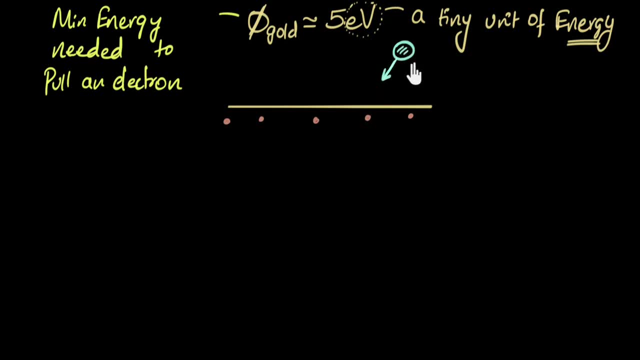 let me draw photon. this is a photon. let's say I shine light whose photon has an energy of 7, 7 electron volt fine. Let's say I shine light whose photon has an energy of 7 electron volt fine. So I shine light whose photons have seven electron volts. 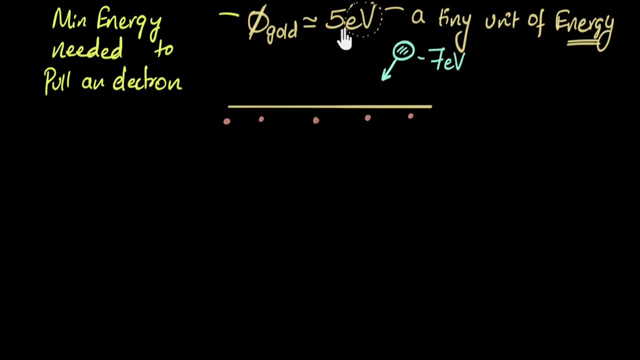 of energy. I know the minimum energy needed to pull this electron is five electron volt. The important part is the minimum over here. My question to you is: what energies do you think, with what energy do you think the electrons will come out? 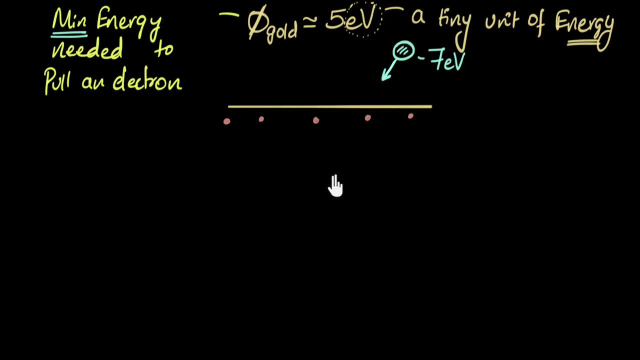 What will be their kinetic energy when they come out of this metal? I want you to pause the video and think a little bit about it. What do you think? what would your answer be? All right, I would think: look, I know to remove this electron out of the metal. 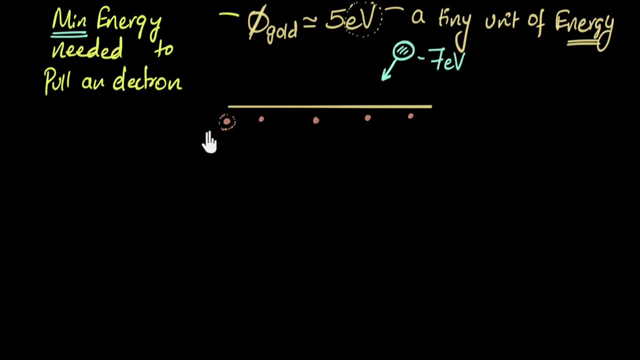 it takes five electron volts of energy. So when it absorbs seven electron volt it has more than energy needed. So it will use up five to escape, And then the leftover two comes out as kinetic energy, because energy is conserved. So that's my answer. 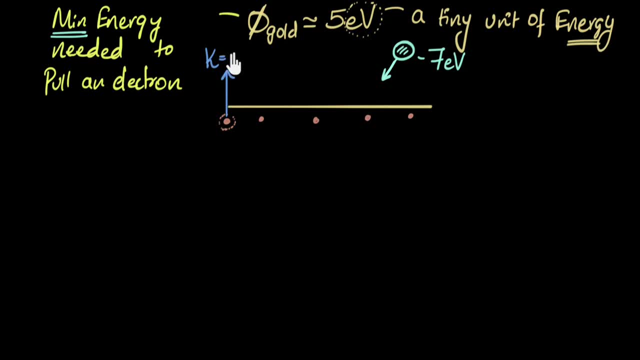 That's what I usually think. So this electron must be coming out with two electron volts of kinetic energy, And that's certainly possible. But there are many other things possible as well. Let me give you another example of what can happen. Let's say this electron. pretty much the same story. 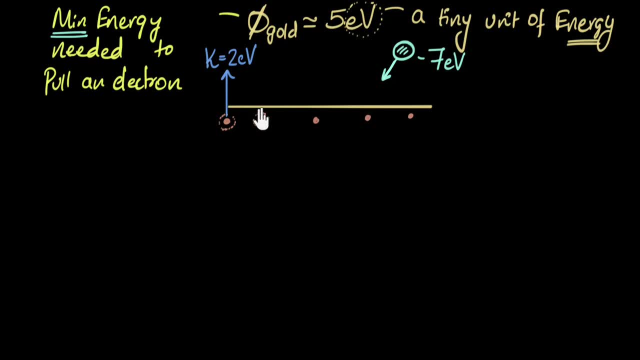 Let's say this: electron also requires five electron volts of energy to escape. It absorbs, it uses five to escape. It only needs five to escape. So the remaining two comes out as kinetic energy. But let's say, while it is moving up. 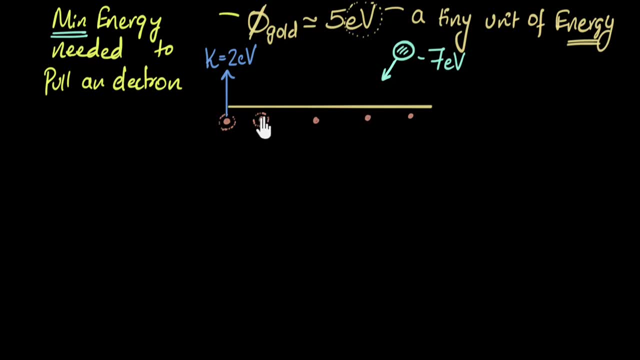 it collides with some of the electrons and loses energy, Then out of two it would have lost some energy, And so this electron will not come out with two. Maybe it only comes out with- I don't know- maybe 1.5 electron volts of energy. 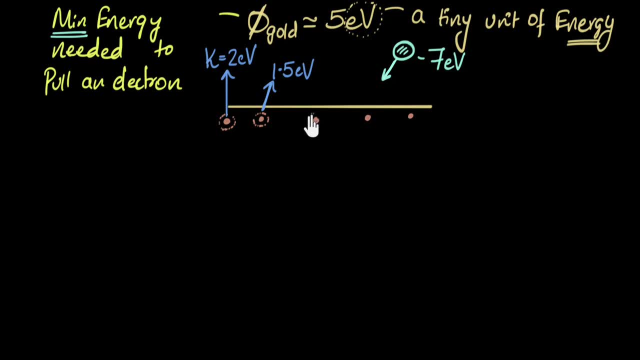 That's completely possible. Maybe when this one absorbs seven electron volts, and when it is coming out, maybe it collides with so many electrons, Maybe so it got so unlucky that, let's say, it lost all its kinetic energy, And so maybe it doesn't come out at all. 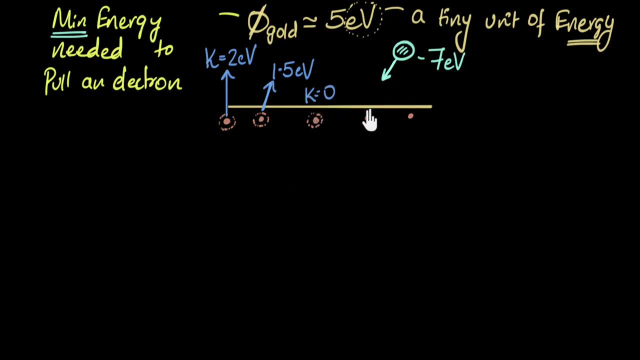 That's also possible. And there's another case possible: Maybe this electron is more tightly bound to the gold nucleus And therefore maybe this one needs six electron volts to escape. You might say: wait a second. you said you know gold requires five electron volts. 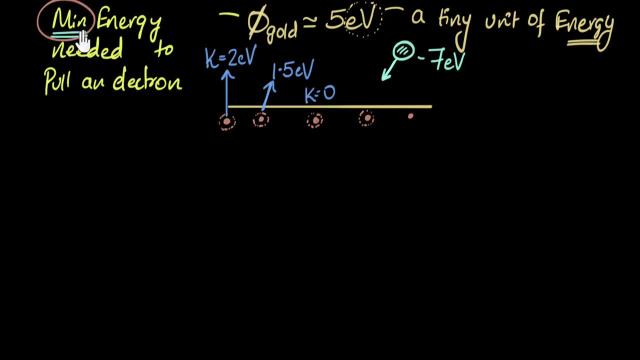 And that's what I want you to remember. It's the minimum energy. Some electrons will need more than that. See, the way to read this is: at least five is needed to pull an electron out, But some electrons would require more than that. 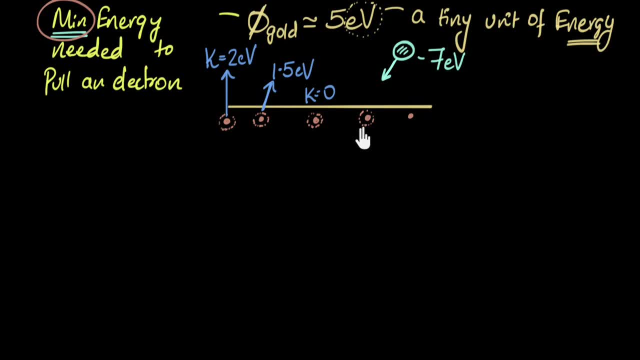 So maybe this one requires six to pull out, And when it absorbs it uses six And only one is remaining, And maybe it got lucky it did not collide. So then it'll come out with kinetic energy of one electron volt, And so on and so forth. 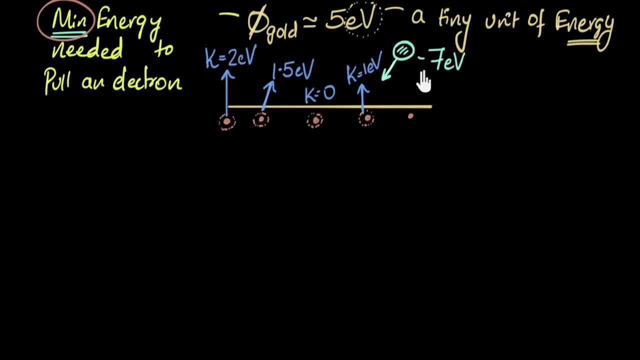 Do you think any electron in this situation for gold, when you shine seven electron volts of light, do you think any electron can come with more energy than two electron volts? Can someone have more than two? I want you to pause and think a little bit about it. 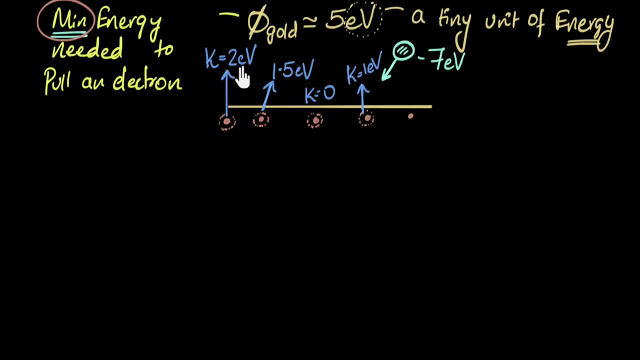 Do you think that's possible? No, It's not possible, because I know for sure that any electron I take, you have to at least spend five from this to escape. You can spend more, But you at least need to spend five. So if I at least spend five, 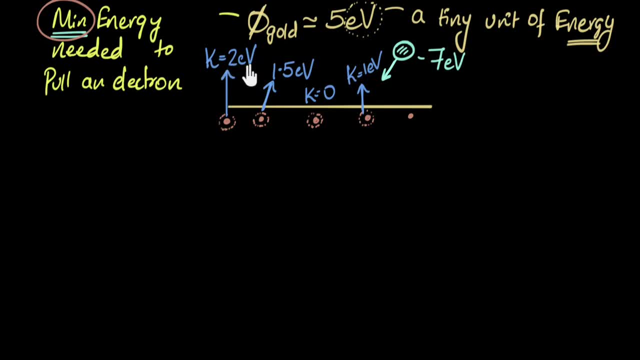 the maximum available energy for kinetic energy is two. It can be less also, but you cannot have more than two, And therefore I know that in this situation this is the maximum kinetic energy available. So, given this value and given the energy of the photon, 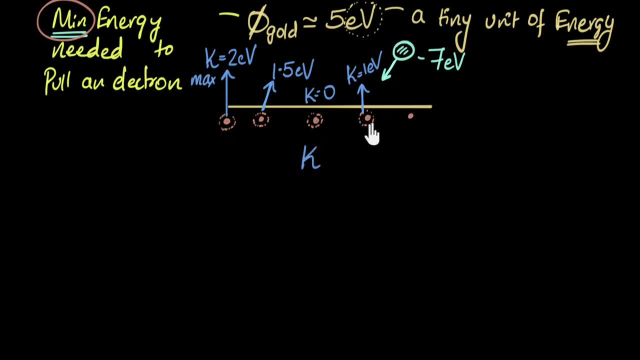 I now can tell that the kinetic energies of the electrons that are coming out will be a range. It will be between zero, because zero is totally possible, and I know the maximum value is two electron volt. And now we see in photoelectric effect. 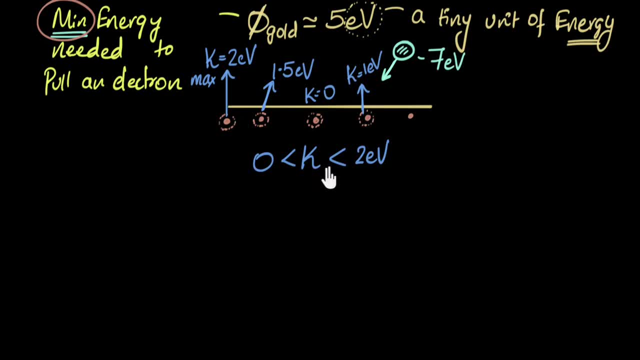 why electrons don't just come out with a single energy. there's a whole spectrum of it, The main reason being because electrons can be more or less tightly bound, requiring more or less energy to escape, and electrons can also collide on its way out. 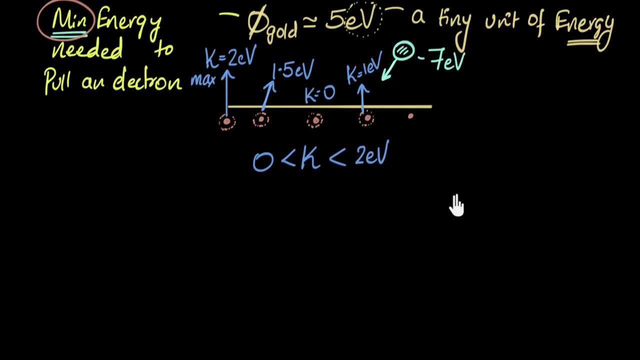 and can lose energy. Now just to check our understanding, let's do one more quick, quick problem. Let's say we take the metal cesium. It turns out that the work function of cesium is somewhere around two electron volt. And let's say we shine the same light. 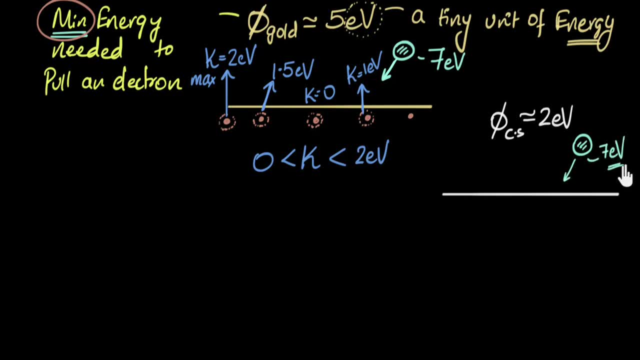 which has the same photon strength, seven electron volt. Can you pause and think about what would be the kinetic energy range over here in this case? All right, I always think about the electron that is the most loosely bound, the luckiest one, which is not gonna collide. 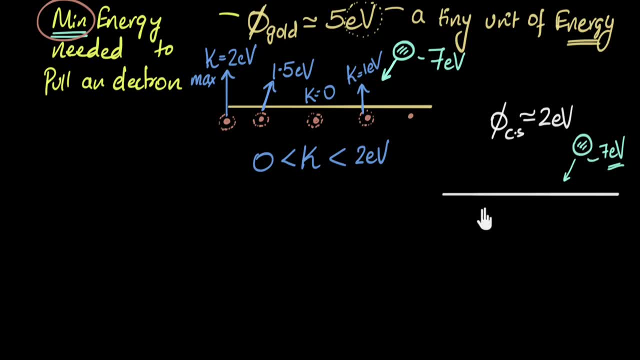 What would happen to that electron? Well, when that electron absorbs the energy- seven electron volts- it will take two to escape. Two is the minimum. That's the minimum. You can't avoid that. It's gonna take two to escape. 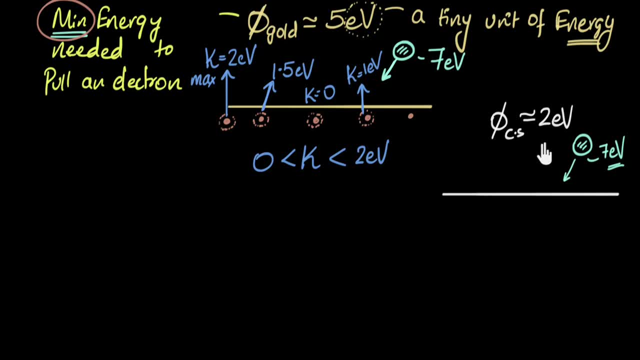 And so the remaining energy would be kinetic energy would be five, But I know that other electrons may not be so lucky, and so we can have anything between zero and five. So immediately I now know that the kinetic energy in this case is gonna be between zero and five electron volt. 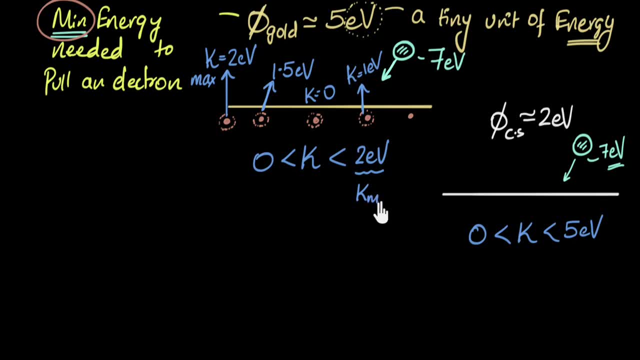 And so the final question I have for you is: since this is the maximum kinetic energy, this represents maximum kinetic energy. the final question I have for you is: what is the connection between the maximum kinetic energy and the maximum kinetic energy? And so the final question I have for you is: 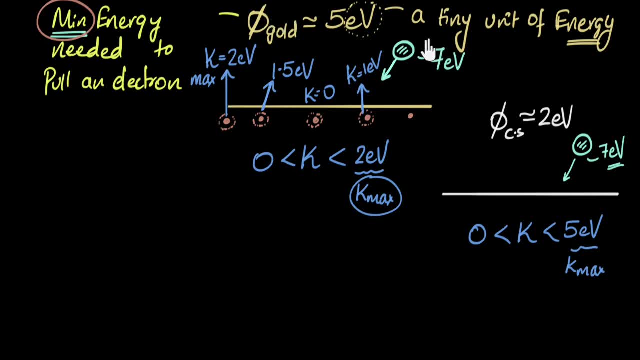 what is the connection between the maximum kinetic energy, the work function and the energy of the photon? Can you, based on whatever you just learned, can you come up with an expression that connects them? We see that the maximum kinetic energy always happens to be the energy of the photon. 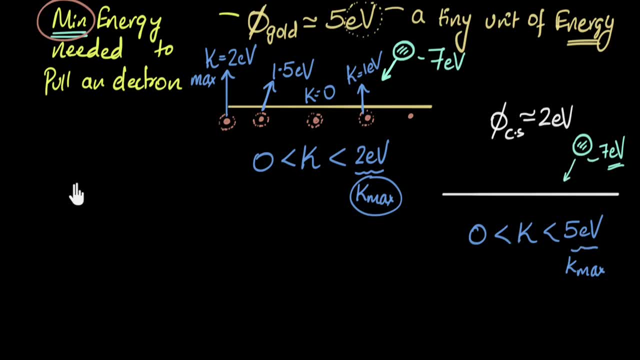 minus the work function. Can you see that? That's how we got that, So let me write that down. The maximum kinetic energy of an electron in photoelectric effect happens to be the energy of the photon minus the work function. Work function. 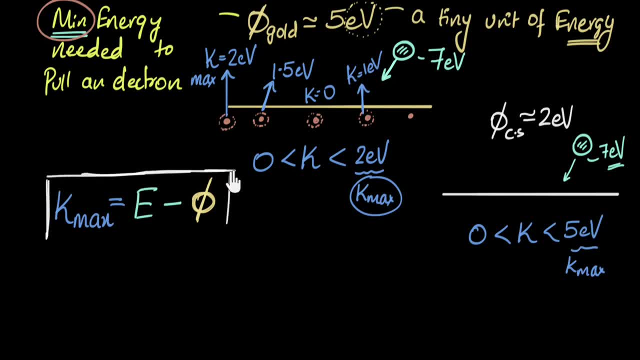 And this is the famous Einstein's photoelectric equation which won him the Nobel Prize. And you may be wondering: hey, we also came up with this equation. Yeah, but we knew about photons and all of that. He had to come up with all of this himself. 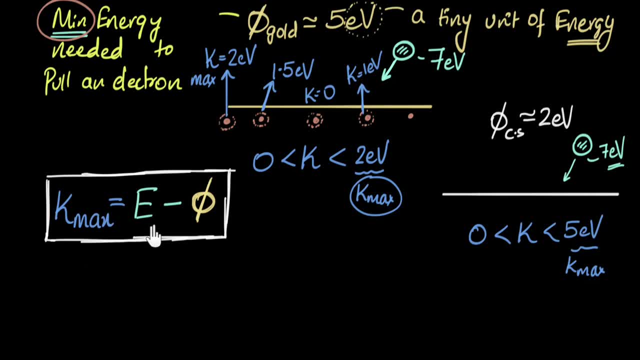 But what I love is that it's not very complex equation or something. It's a simple, elegant looking equation which is able to explain amazing things that couldn't be explained back in the 1900s. But the important thing to stress on is: